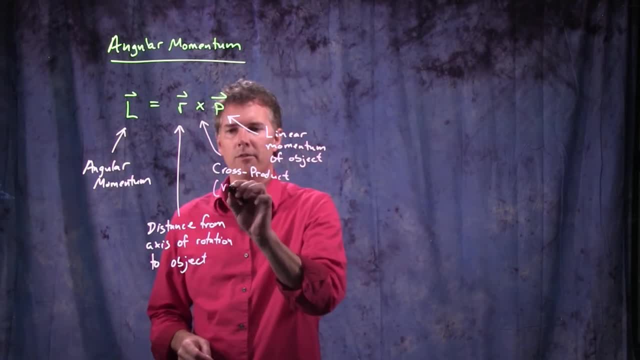 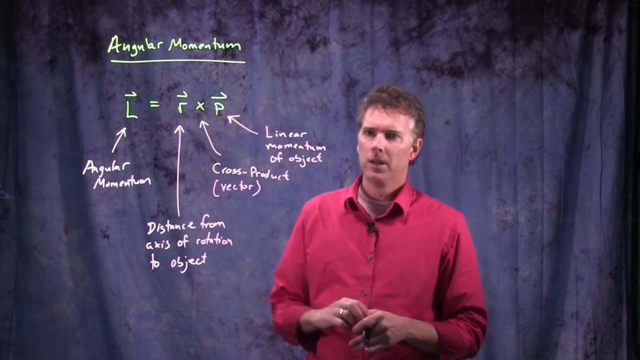 us a scalar, But now the cross product is in fact a vector quantity, And that's why the L has a vector on top of it, over on the left side. So this is what we need to understand, And let's identify first what the cross product is and then 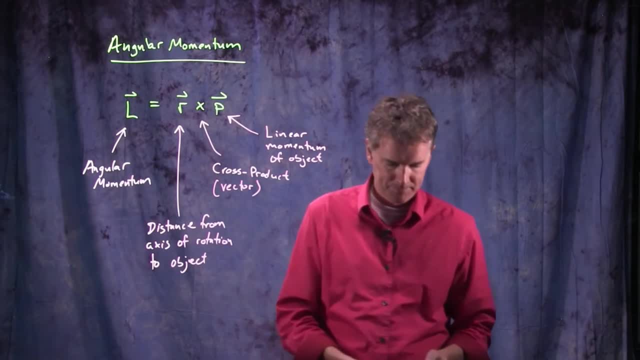 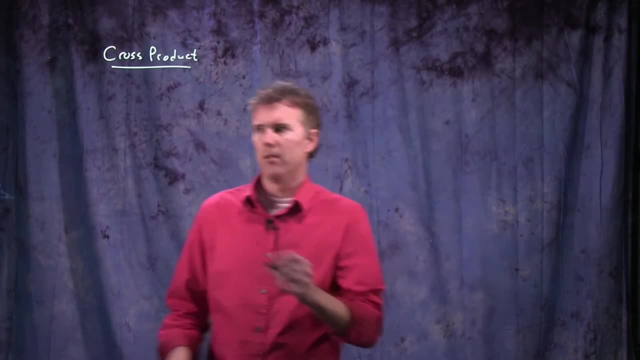 how to apply it to various angular momentum problems. Okay, what is this cross product that we're talking about? The cross product is the following. Let's say, I have vector A and it looks like this, And I have vector B and it looks like this. 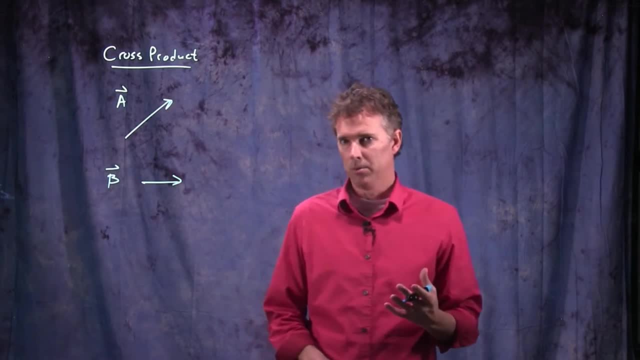 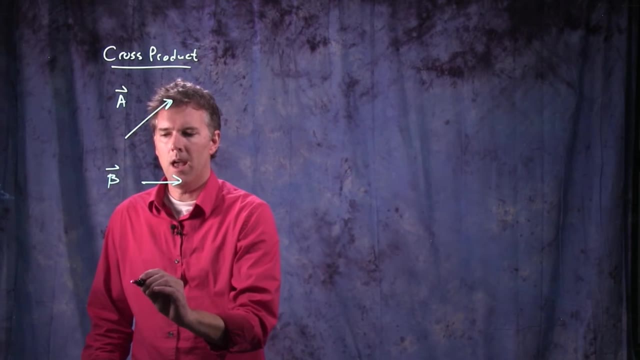 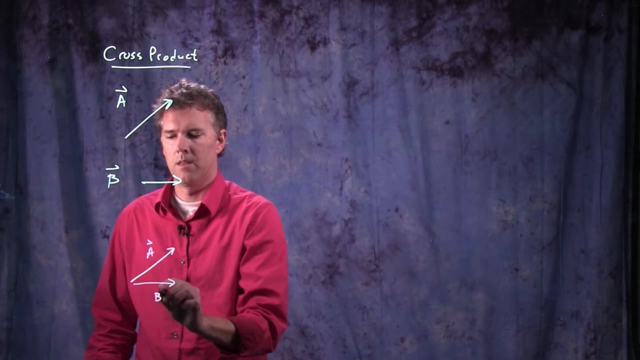 It looks like that And I want to figure out the cross product between these two, not the dot product. The way you figure it out is you put them together, A and B, And then you figure out what the angle is between them, And we're going to call that angle phi Before. 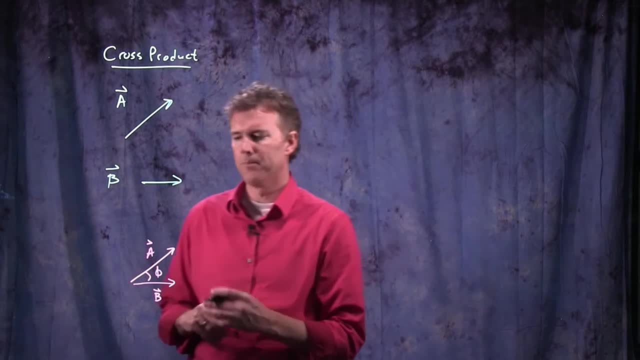 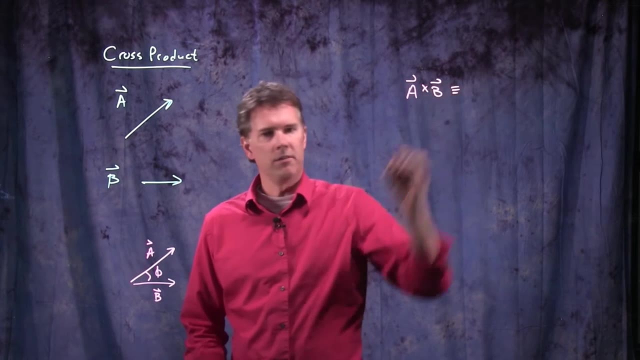 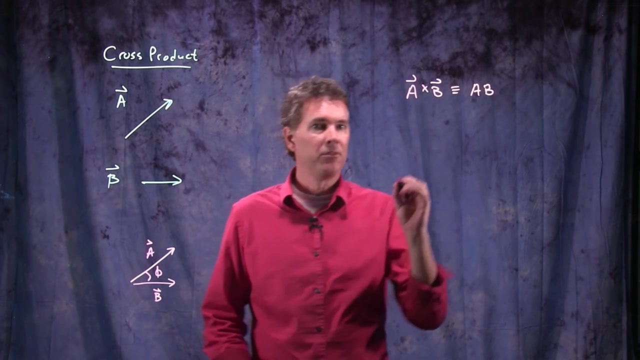 when we did the dot product we called it theta, So in this case we'll call it phi. The cross product A cross B is defined as the following: It's magnitude of A times magnitude of B times the sine of the angle between them. Remember when we did the dot product we had cosine. 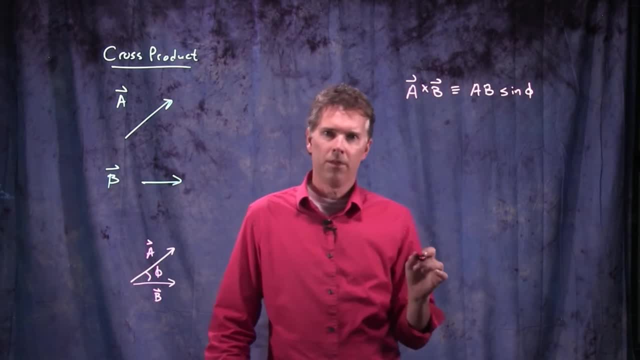 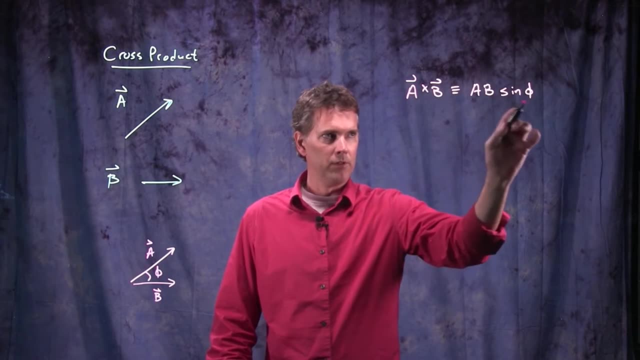 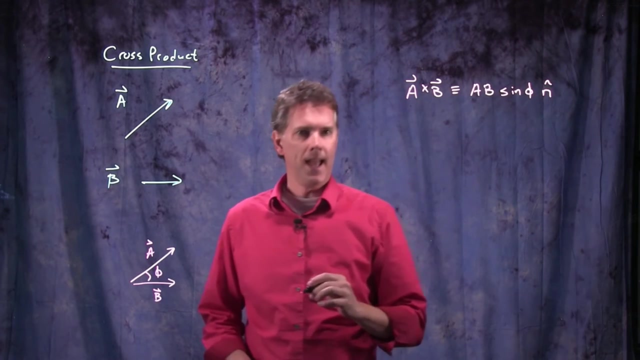 Now, it's the sine of the angle between them. But there's one more thing that's really important here, which is cross product is a vector quantity. This that we've written so far is just a magnitude, And so we need to identify a direction, And so, for the direction, we do an N-hat right there. 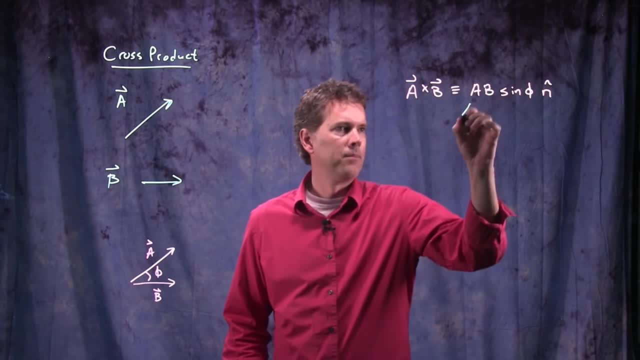 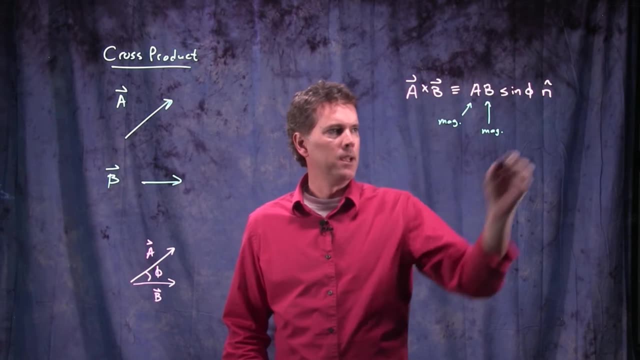 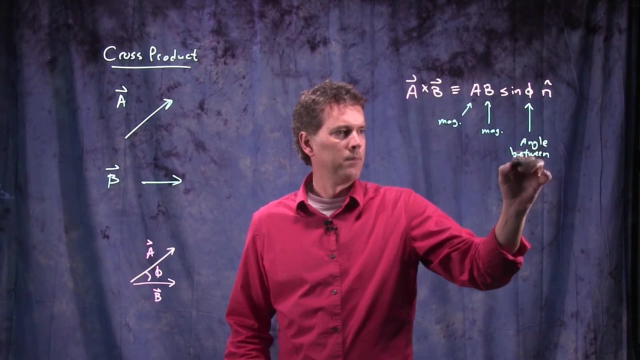 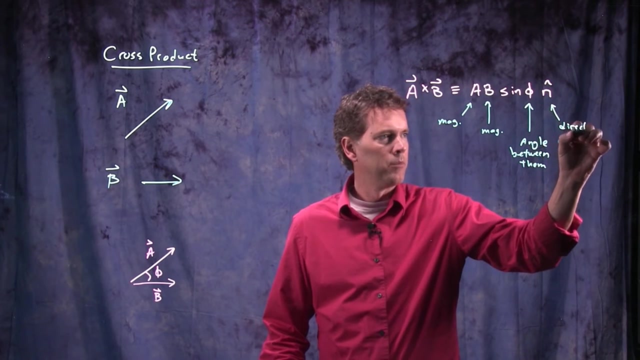 This is, of course, the magnitude of vector A, This is the magnitude of vector B, This is the angle between them And this is the resultant direction which we need to figure out from something called the right-hand rule. So how do we figure out this direction? 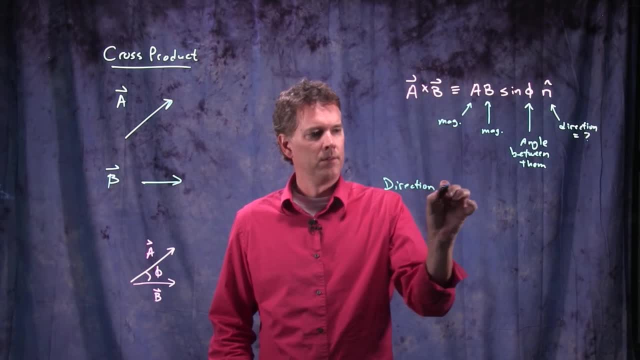 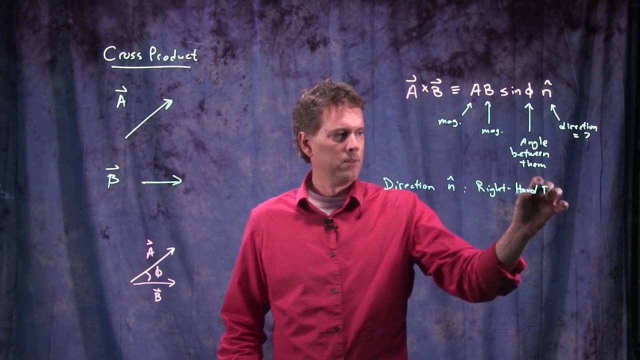 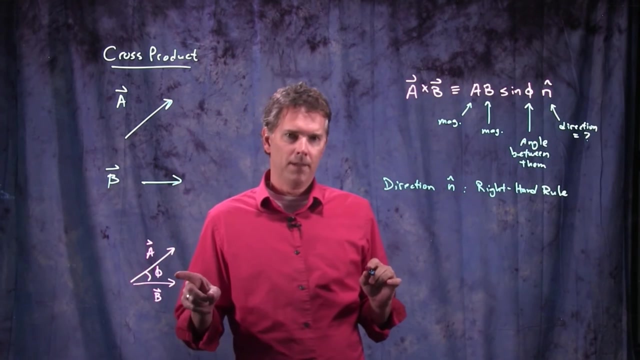 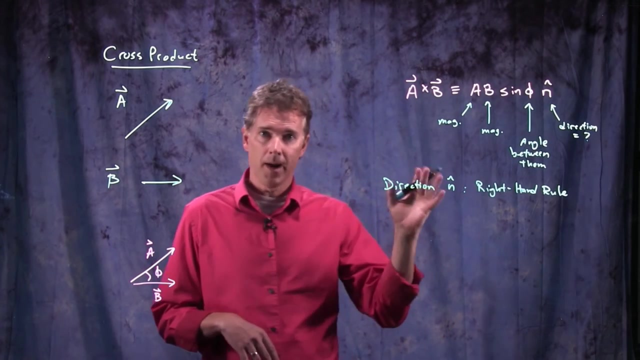 The direction. n-hat, we follow what's called the right-hand rule. Okay, If I have vector a and vector b, I can figure out the direction of the cross product if I'm very careful about following the right-hand rule. Now, this is a little tricky with the learning glass because my right hand is looking like left-hand to you. 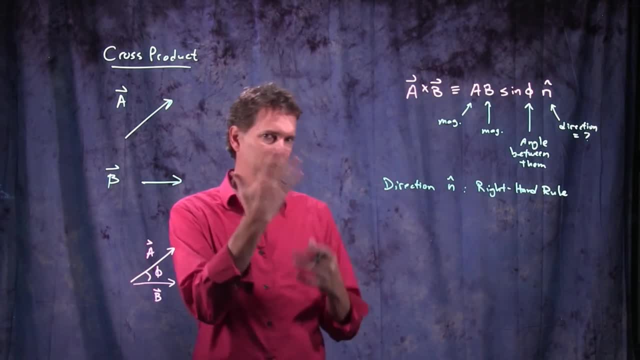 So I in fact have to use my left hand. You'll notice that the ring is on this hand, So it's really my left hand, even though it looks like my right hand to you guys. The right-hand rule is the following: 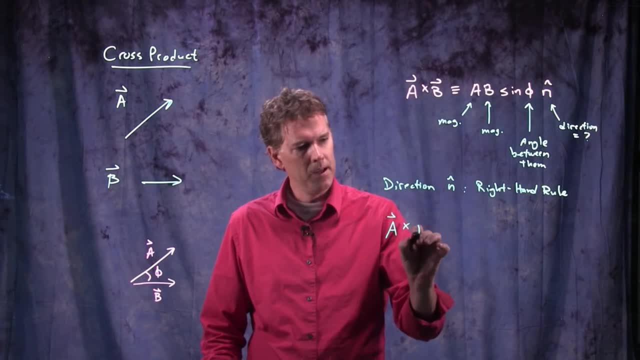 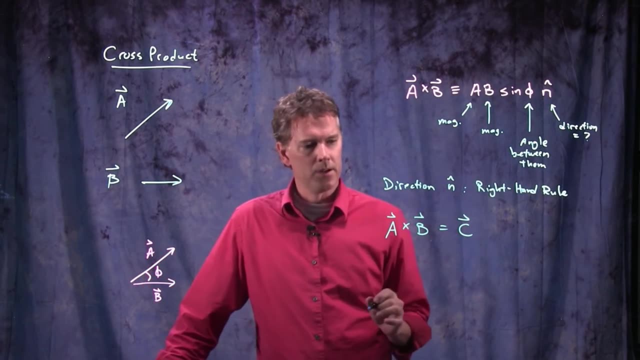 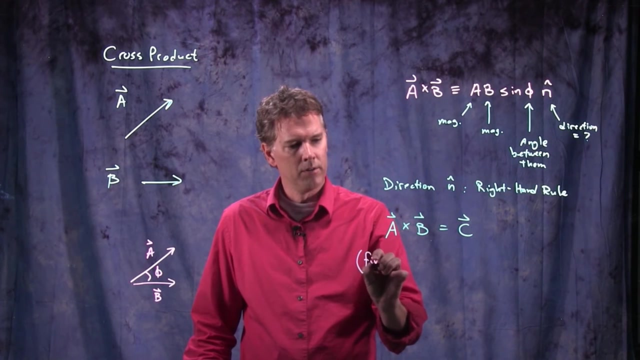 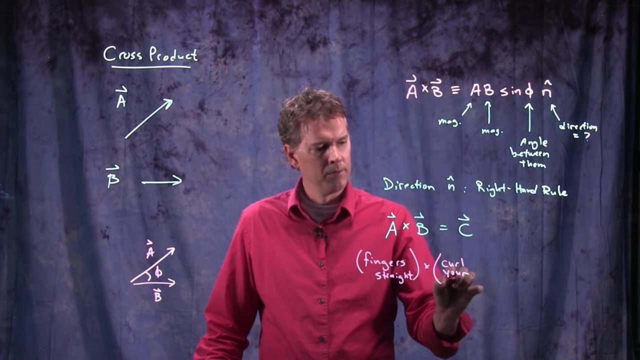 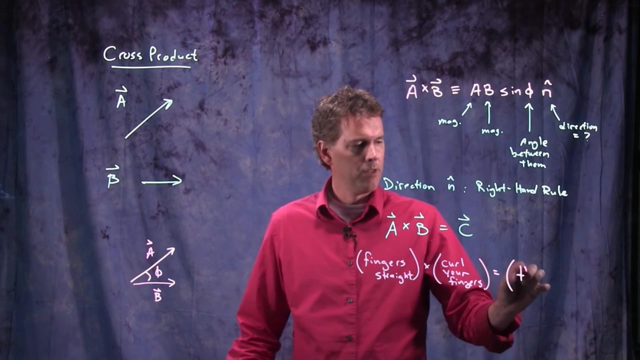 If I have a cross b and that's going to equal some vector c, the way you figure out the direction is the following: A- you do your fingers straight. B is you curl your fingers. C is the direction of your thumb. 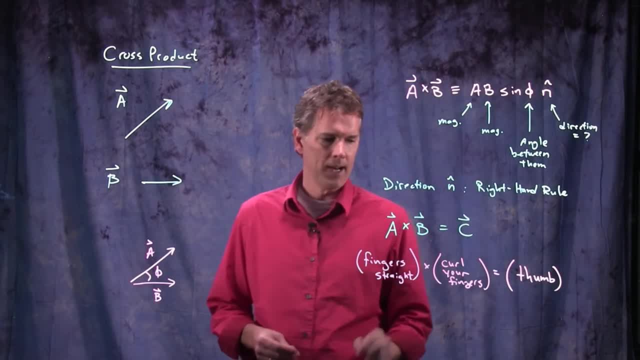 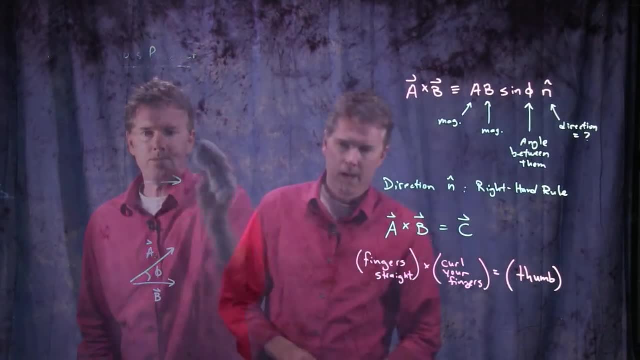 And it's called the right-hand rule Because you have to do it with your right hand. So let's see if we can figure it out for this simple example that we just talked about. Okay, if we just have two vectors- and I'm going to change the order slightly- 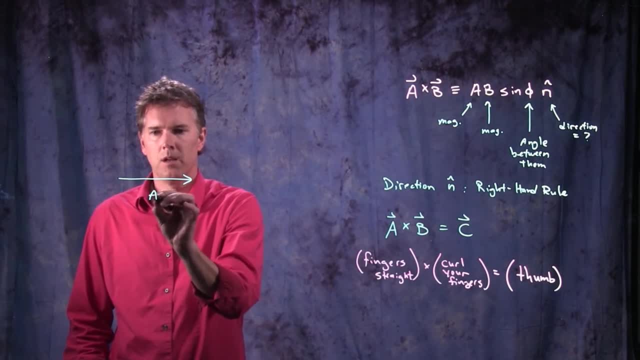 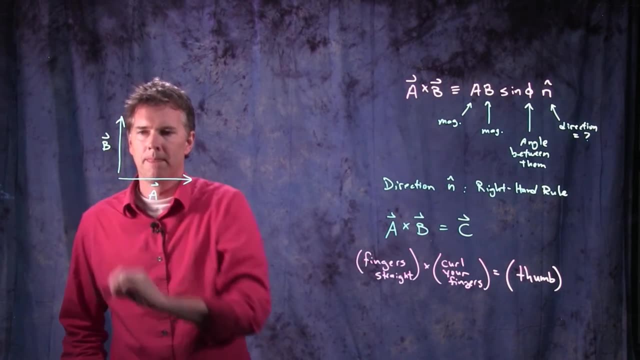 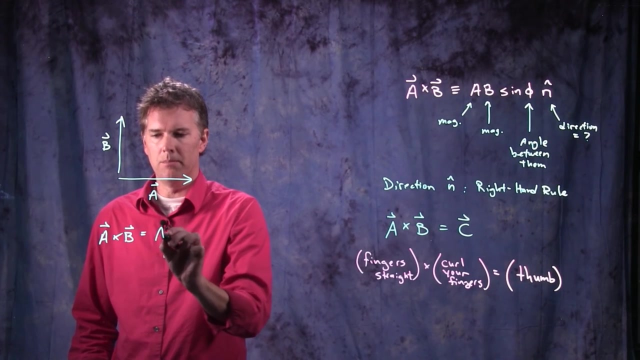 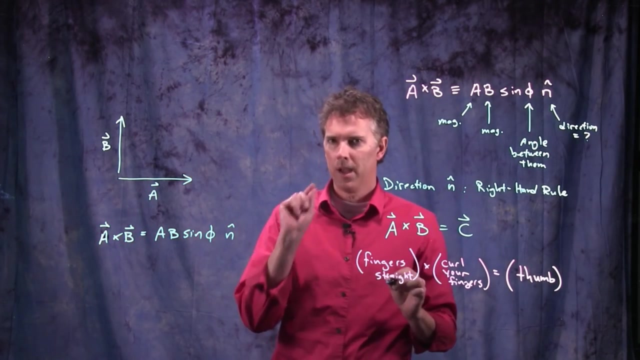 Let's say we have vector a pointing to the right And we have vector b pointing up. What is a cross b? Okay, A cross b, It's going to be magnitude of a, magnitude of b times the sine of the angle between them with a particular direction. 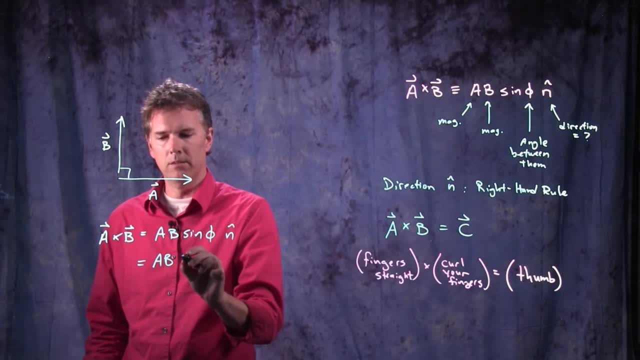 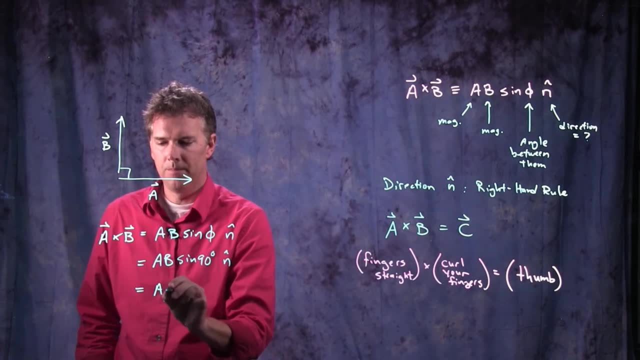 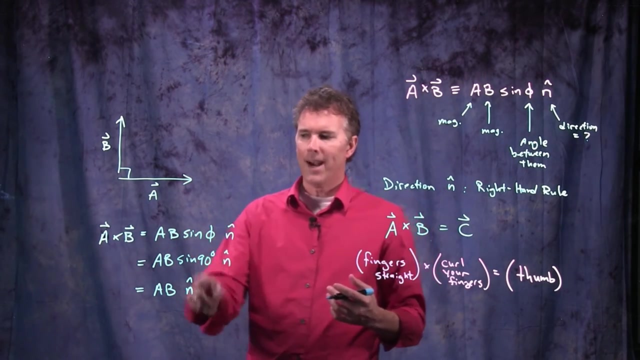 But the angle between these two is a right angle, And so we get sine of 90 degrees, And so we just get ab and hat. Sine of 90 degrees is, of course, one. Now, how do we figure out the direction for this thing? 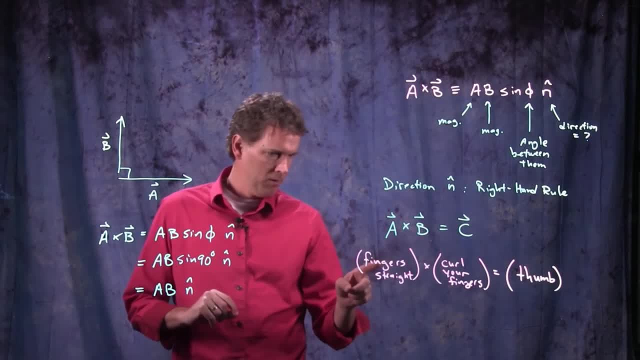 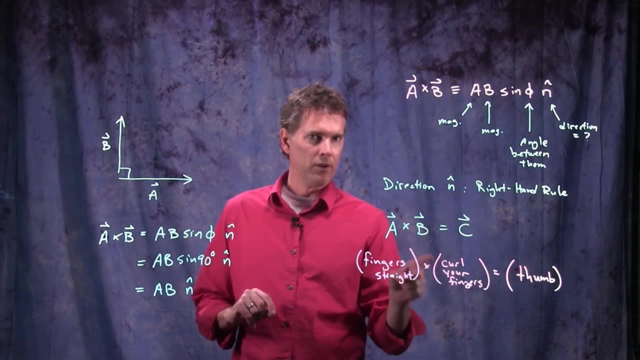 Okay, Which way? Which way is it going? Well, what we said over here was, if I do my fingers straight in the direction of a and then I do my fingers curled in the direction of b, that should be the direction for c, which is given by my thumb.